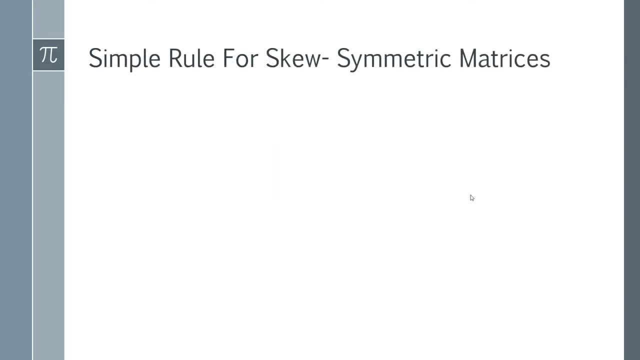 case of a skew symmetric matrix, you have a similarly simple rule, with a slight change. so a matrix is skew symmetric if a transpose is equal to the negative of your matrix, a. so if you find the transpose of a and it's equal to exactly the negative by every single element of your 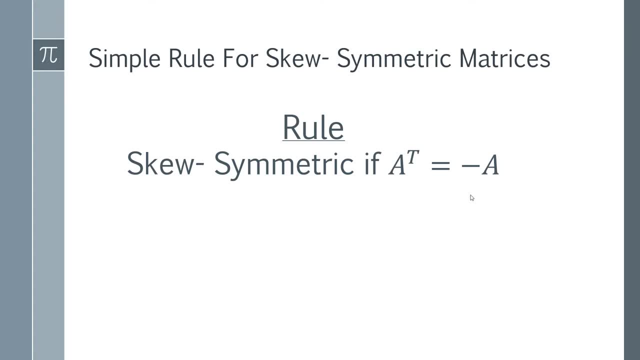 original matrix a. you have a skew symmetric matrix and you can actually use two quite simple and quick visual checks to see if a matrix has a chance of being skew symmetric. so let's look at this matrix here. so, firstly, in order to be skew symmetric, you must have a square matrix, non-square. 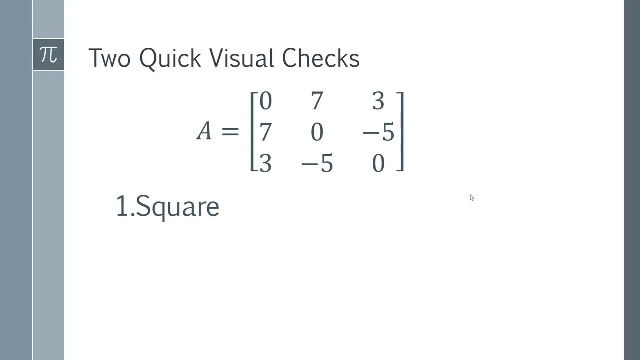 matrices are never going to be skew symmetric. so if it's non-square, just immediately don't bother doing any proof, just say it's not skew symmetric, because it isn't going to be. the second one is that the least leading diagonals must be zero. so if you have any numbers on these leading diagonals, it's going to. 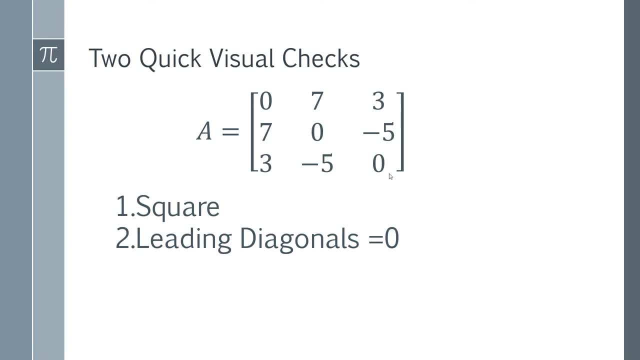 immediately tell you that that matrix is not going to be skew symmetric because when you find the transpose, these elements don't actually change position, so they're not going to switch signs. so you're not going to have a skew symmetric matrix. so let's look at this in practice and just look. 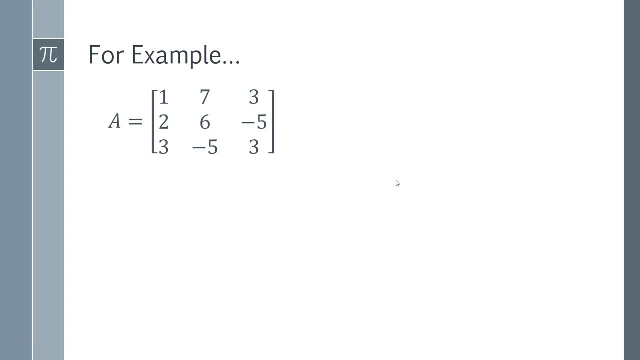 at some simple examples that we can immediately tell if they're skew symmetric or not. the first one: immediately: not skew symmetric. leading diagonals, not all zero, therefore can't be skew symmetric. in the second case, we've got a similar matrix again, immediately can tell the leading diagonals are wrong. can't be skew symmetric. we look at this one. 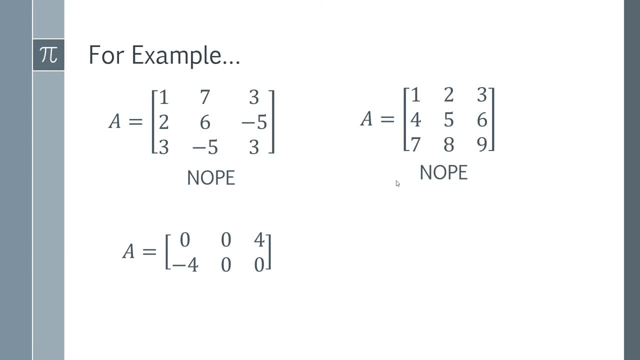 it looks a bit better, but it's a non-square matrix, so it's not going to be skew symmetric. so we can say nope, that one's not skew symmetric. the next one: we've got the leading diagonals that are zero and we've got square matrix. this one has a chance of being skew symmetric. so this one you would. 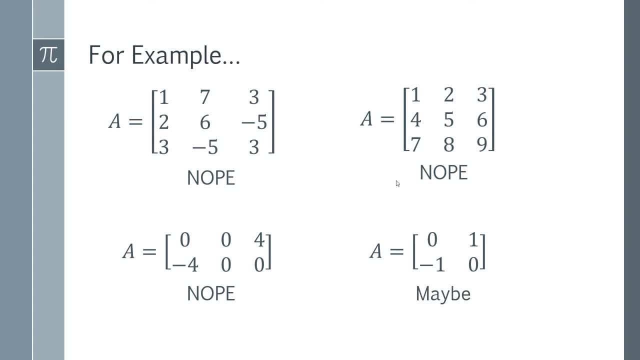 actually have to do the check to see if it was skew symmetric or not. so you see how that visual check you can immediately rule out the vast majority of all matrices that you come across and know that they're not skew symmetric and only focus on those that actually have a chance of being skew symmetric. so let's.